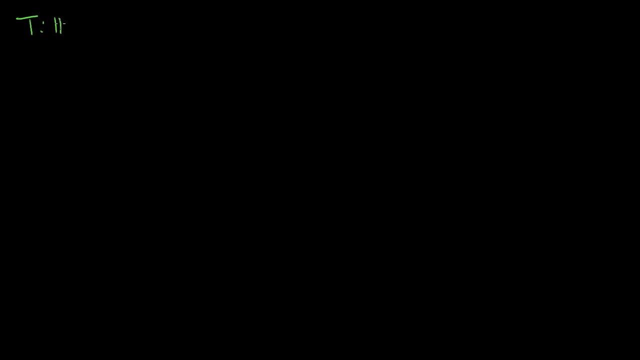 Let's say I have some transformation from R2 to R2. And it's essentially just a multiplication times a matrix, And we know that all linear transformations can be expressed as a multiplication of a matrix. But this one is equal to the matrix 1,, 3,, 2,, 6 times. 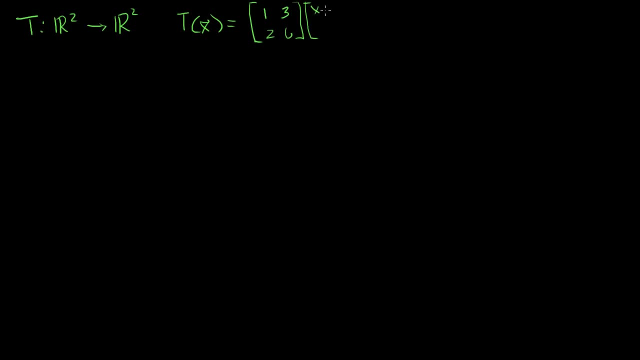 whatever vector you give me in my domain Times x1, x2.. Now let's say I have some subset in my codomain, So let me draw this right here. So my domain looks like that It's R2.. And, of course, my function or my transformation maps. 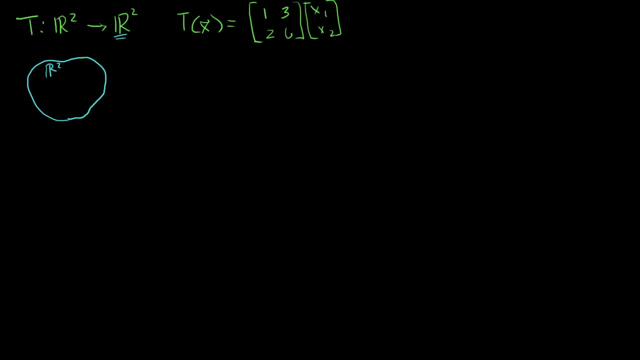 elements of R2 into elements of its codomain, which also happens to be R2.. I could show it mapping into itself, but for the sake of simplicity let's draw my codomain here And our transformation of course maps for any. 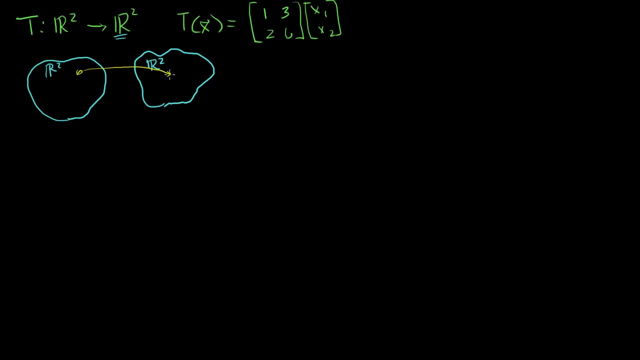 element here. The transformation of that will be an association or a mapping into R2.. Now what if we take some subset of R2, and let's just say it's a set of two vectors: The 0 vector in R2 and the vector 1, 2.. 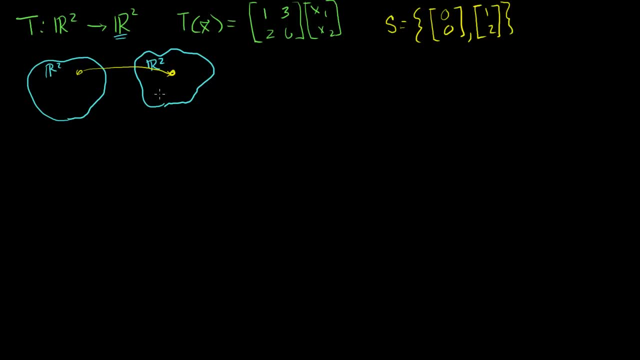 So it's literally. let's say, it's this point. Let me do it in a different color. Let's say: this is my 0 vector in R2.. I'm not plotting them, I'm just showing that they're in R2.. 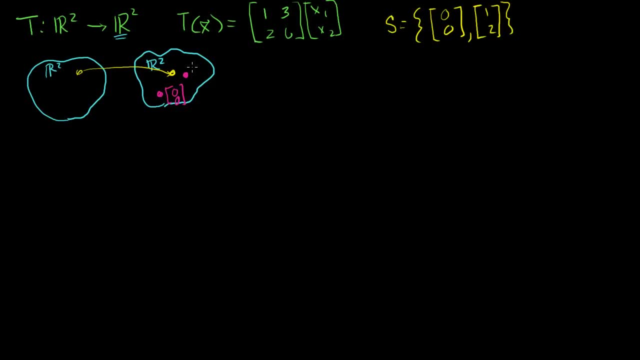 That's my 0 vector And let's say the vector 1, 2 is here 1, 2.. What I want to know is what are all of the vectors in my domain whose transformations map to this subset, map to. 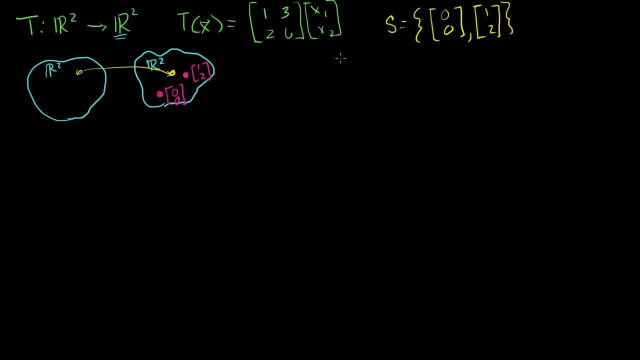 this point. So I want to know the pre-image of S. So the pre-image of S under This is the pre-image of S under T. And I said be careful because when you just say pre-image of something without saying under something else, it implies. 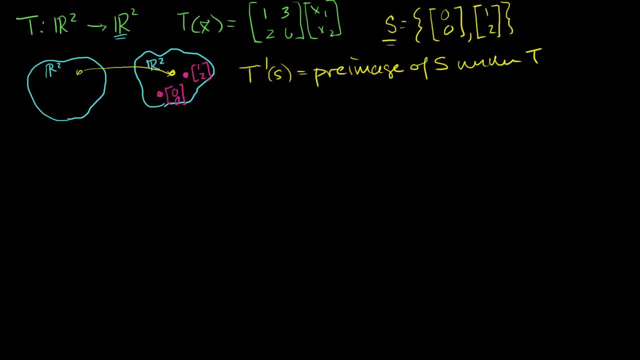 that you're taking. well, when you say image of something, it implies you're taking the image of an entire transformation, like I showed you, I think, two videos ago. But when you're taking the image or pre-image of a set, 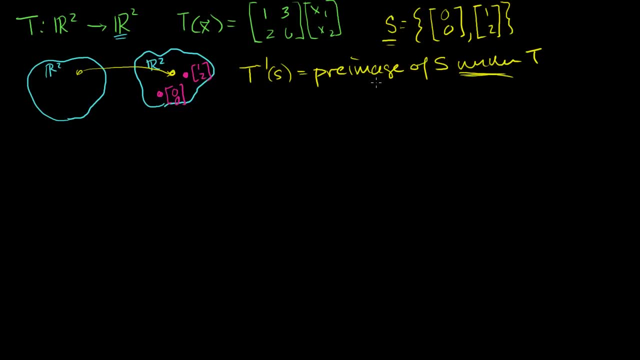 yeah, make sure you say under what transformation. So we want to know the pre-image of this subset of our co-domain under the transformation T, And we write this as T inverse of S, And we saw in the last video. this is all of the elements in 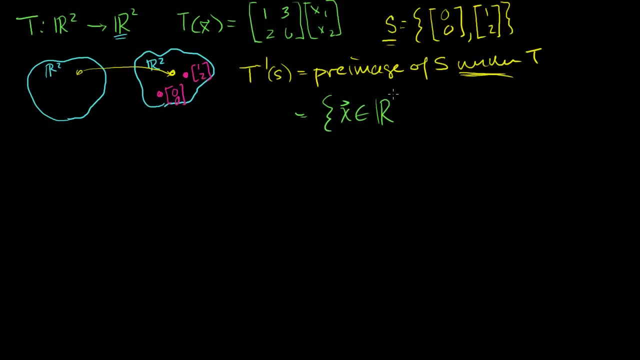 our domain, where the transformation of those X's is a member of the subset of our co-domain that we're trying to find the pre-image of. Now what is another way of writing this? Well, you could write this as we're trying to look for all of. 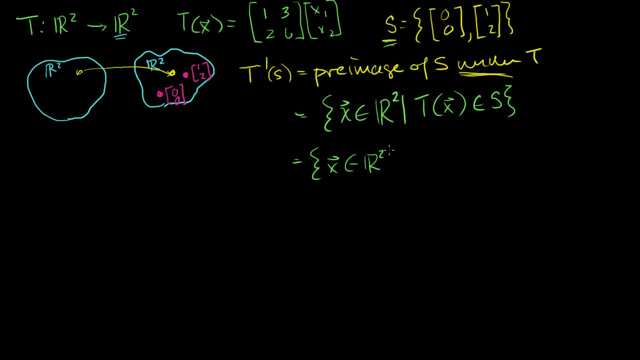 the X's in our domain, such that this vector, let's call this A, That matrix, A, Such that A times X is a member of S. So that means A times X has to be equal to this or has to be equal to that. 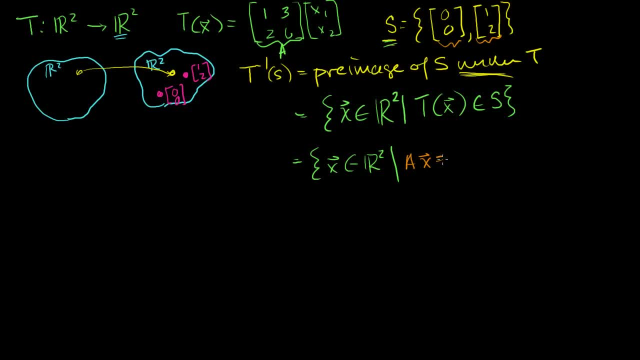 So that means A times our vector X has to be equal to the 0 vector, Or A times our vector X. OK, x has to be equal to this vector 1, 2.. This is the exact same statement as this one, right. 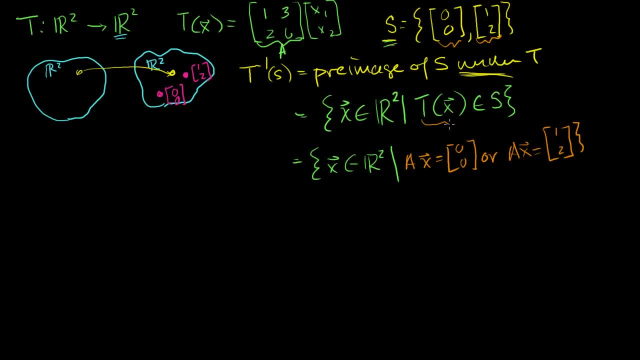 here. I just made it a little bit more explicit in terms of our actual transformation a times x and in terms of what our actual set is. Our set is just two vectors. So if we want to determine the pre-image of s, so we write. 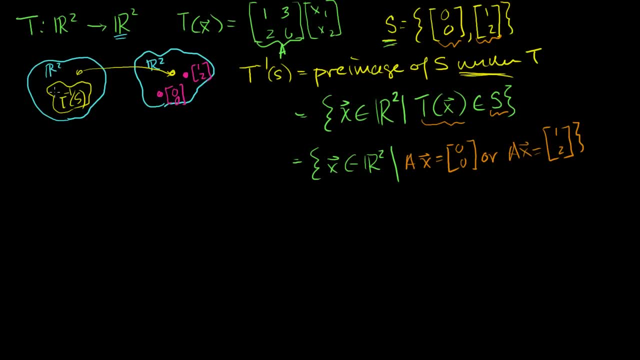 that pre-image of s under t, that set there we essentially have to just find all of the x's that satisfy these two equations right there. So this equation, so we have to find all of the x's that satisfy the first one right here is the matrix 1, 3, 2, 6. 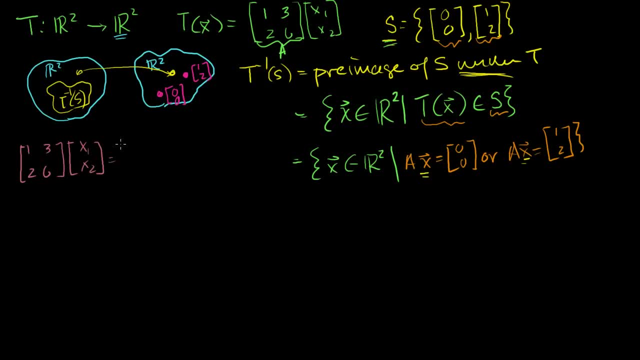 times x1, x2 is equal to the 0 vector. That's this equation, right there, We need to find all of the solutions to that And you might already recognize that, all of the solutions to this, All of the x's. 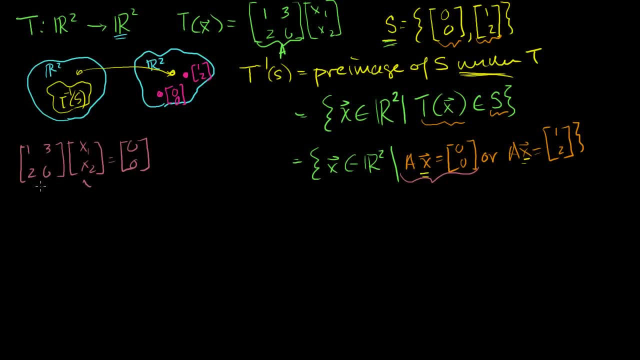 The x's that satisfy. this is the null space of this matrix. I just thought I would point that out on the side. Now, that's not the only one. We also have to solve this guy over here. I'll do that in blue. 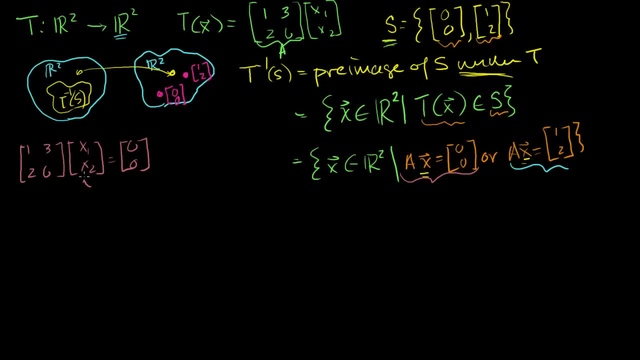 So the pre-image of s under t is going to be all of the solutions to this, plus all of the solutions to 1,, 3,, 2, 6 times x1, x2 is equal to 1, 2.. Now we could just solve this with an augmented matrix. 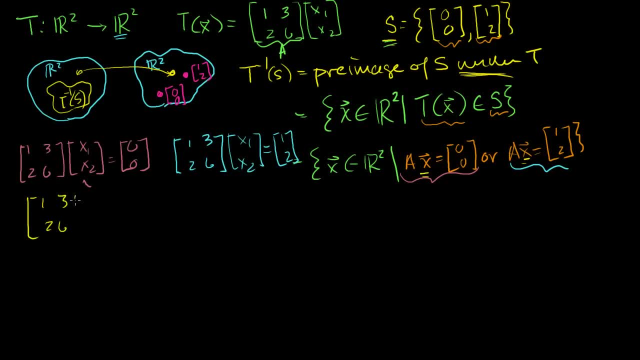 So my augmented matrix would look like 1, 3, 2, 6, 0, 0.. And here my augmented matrix would be 1, 3, 2, 6, 1, 2.. Let's put this in reduced row echelon form. 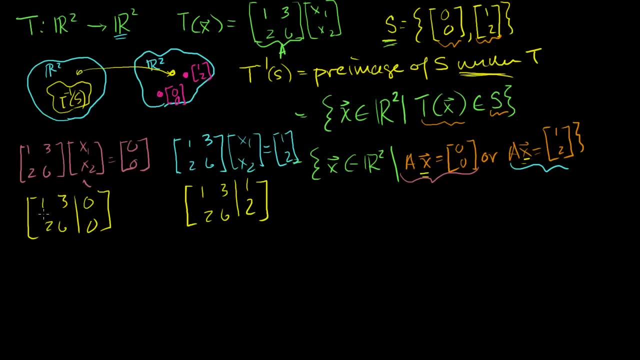 So let's replace our second row with our second row, minus 2 times the first row. So what do we get? Our first row stays the same: 1,, 3, 0.. Let me do them simultaneously. Let me solve these systems in parallel. 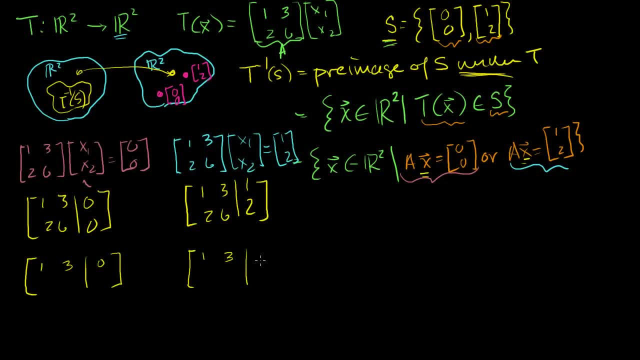 So my first row stays the same: 1,, 3,, 1.. And in both cases, because I just want to get the left-hand side of my augmented matrix into reduced row echelon form, I can apply the same row operation. 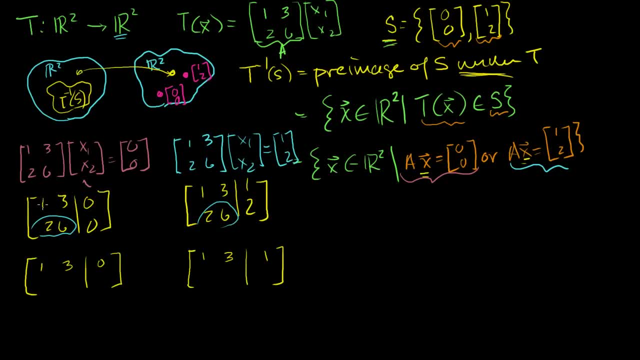 So I'm replacing my second row with 2 times my first row. So 2 minus 2 times 1 is 0.. 6 minus 2 times 3 is 0.. And, of course, 0 minus 2 times 0 is 0.. 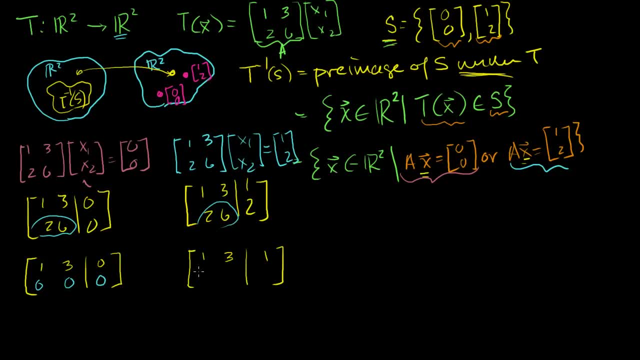 Here: 2 minus 2 times 1 is 0.. 6 minus 2 times 3 is 0. And 2 minus 2 times 1 is 0. So we get all these 0's and we're actually done. 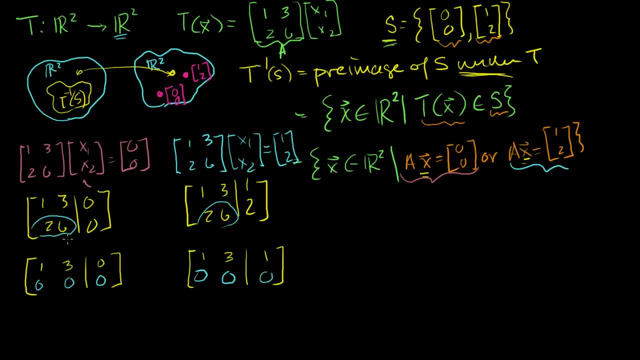 We have both of these augmented matrices in reduced row echelon form, And how do we go back to solve all of the x1's and x2's that satisfy these? Well, you recognize that our first columns right here are pivot columns And these are associated with our variable x1.. 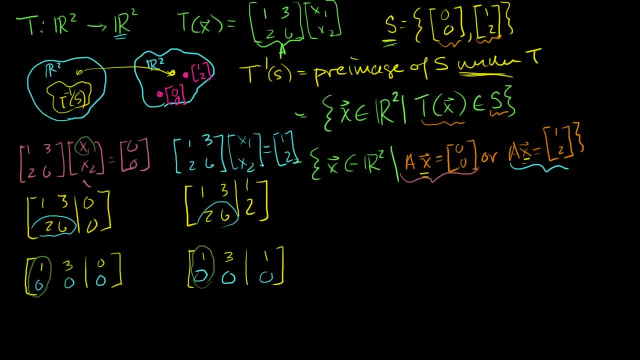 So we know that x1 is the pivot column, So we know that x1 is the pivot column, So we know that x1 is the pivot column, So we know that x1 is a pivot variable And we know that the second column is a non-pivot column. 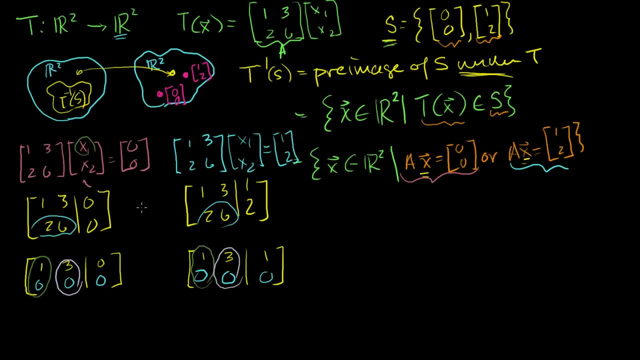 because it has no 1's in it, And so it's associated with x2.. And since x2 isn't a pivot column, we know that x2 is a free variable, which essentially means we can set x2 to be anything. 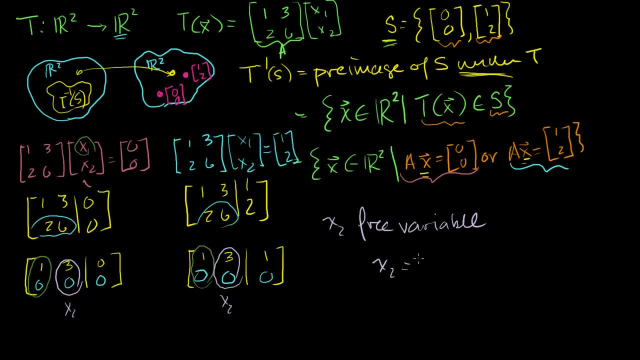 So let's just set x2.. x2 is equal to t, where t is a member of the reals. In this case, what is x1 going to be equal to? So here this top equation says: let me write it: 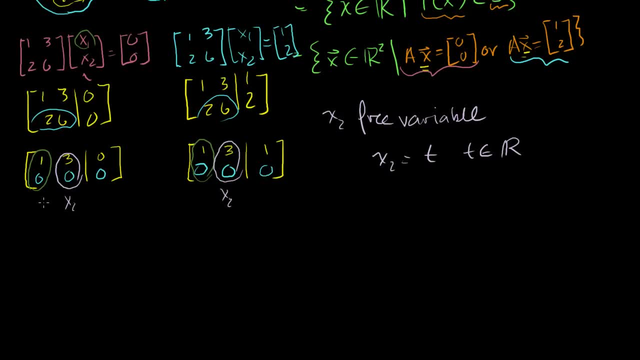 If we just kind of go back to this world right here, this means that x1 plus 3x2 is equal to this 0 here. This top line right here says: x1 plus 3x2 is equal to 1.. And so if we say x2 is equal to t, this equation- 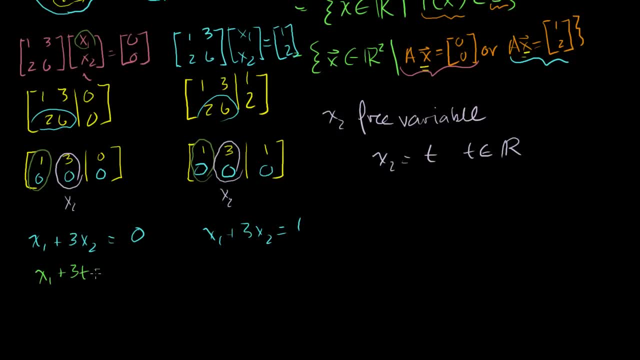 becomes: x1 plus 3t is equal to 0. Subtract 3t from both sides, You get x1 is equal to minus 3t. And then this equation you get x1 is equal to. if we substitute x2 with t is: x1 is equal to 1 minus 3t. 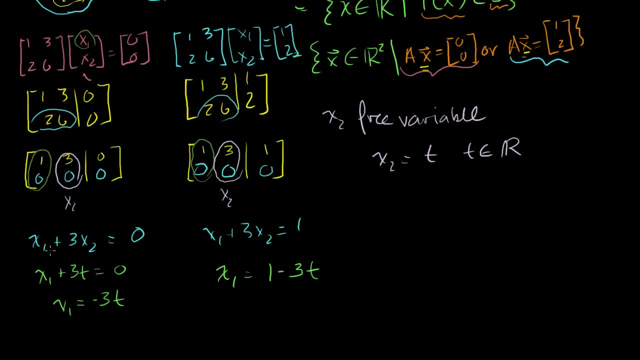 Now if we wanted to write the solution sets in kind of vector notation, the solution set for this guy right here, for this first equation right there, is going to be: x1, x2 is equal to what It's going to be equal to. you have your, it's going to be. 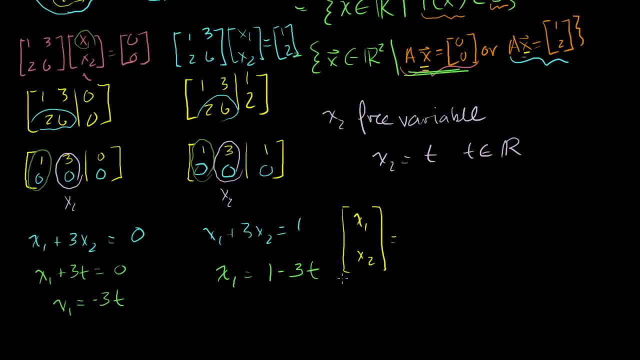 equal to: well, x2 is just going to be equal to t times. it's just going to be equal to t, So let me just write it there. So it's going to be equal to t times. x2 is just t times 1.. 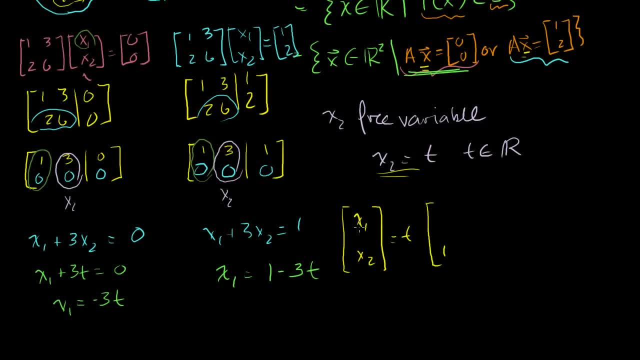 It's just equal to t. I made that definition up here. And then what's x1 equal to? It's equal to minus 3 times t. So if I put a t out here as a scalar, it's just minus 3 times. 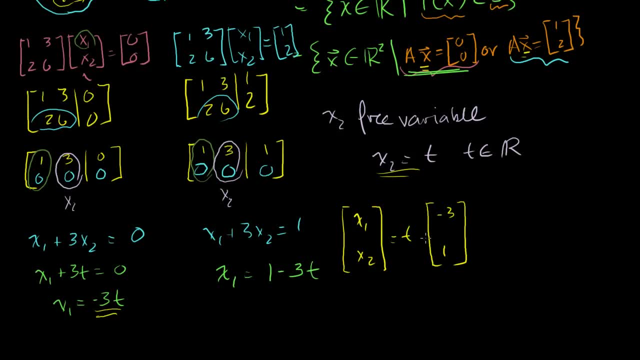 t. So this a solution for this first equation- somewhere where t is a member of the reals. So it's just scalar multiples of the vector minus 3, 1.. And if we think of this as a position vector, this will be a: 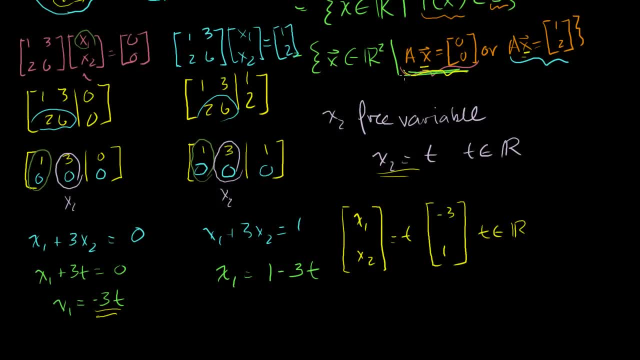 line in R2.. And I'll draw that in a second. So that's the solution for this first equation, And then the solution for the second equation. the solution for this equation. Let me paint this out. Okay, the second equation: how can we set this up? 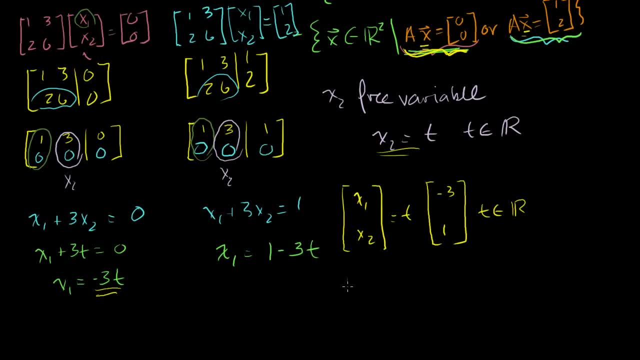 It's going to be. let me make sure you can see it: it is x1,, x2, and let's see x2,, once again, is just t times 1.. So let me just write it like this: So it's t times 1.. 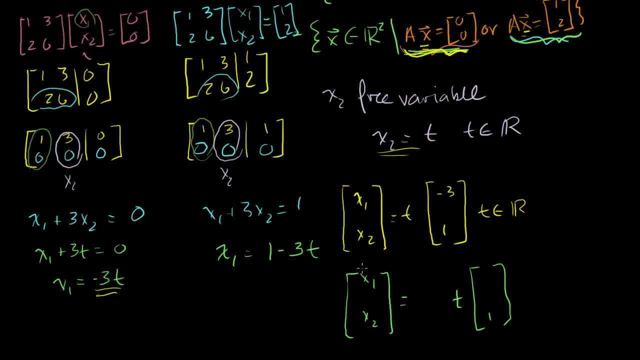 That's x2.. Now what's x1?? x1 is equal to 1 minus 3 times t. So if we do a minus 3, that gives us our minus 3 times t, but we need to do a 1 minus that, or 1 plus minus 3 times. 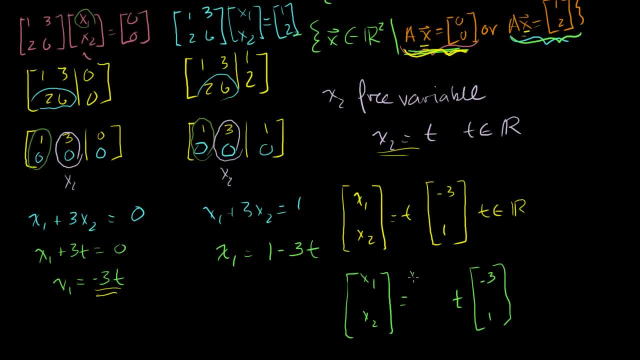 t. so what we can do is we could say that all the solution set here is equal to the vector 1 here. So now we have 1 plus minus 3 times t for x1, and then here we could say is 0.. 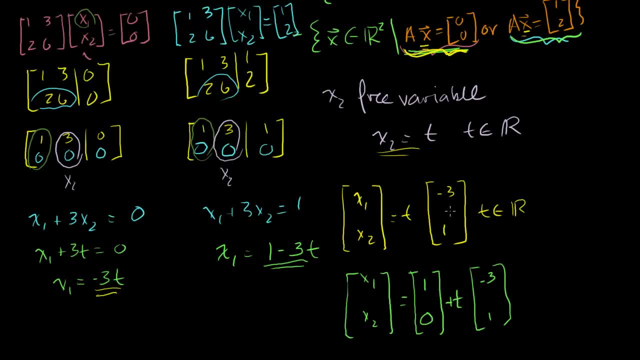 x2 is equal to 0 plus t or x2 is equal to t. So this is the solution set for the second, For the second equation. So our preimage of S- and remember S- was just these two points in our co-domain. 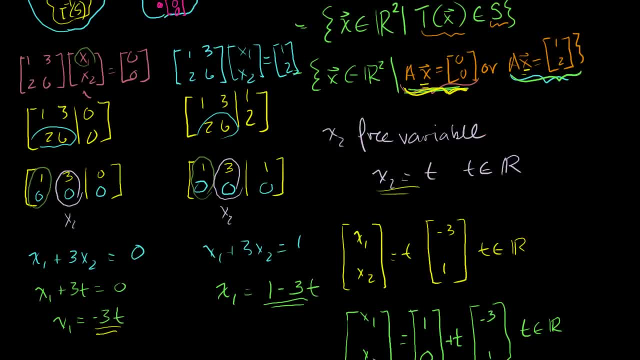 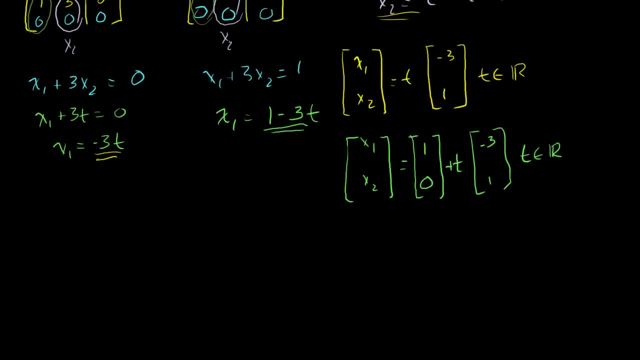 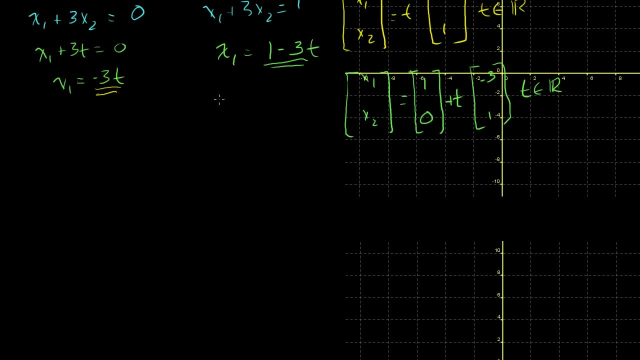 The preimage of S under t is essentially all of the x's that satisfy these two equations, And let's actually graph those. Let me turn on my graphs. That makes it look a little bit messy, but let me graph it down here. 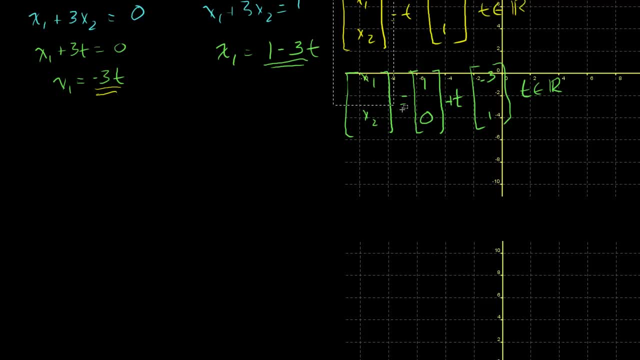 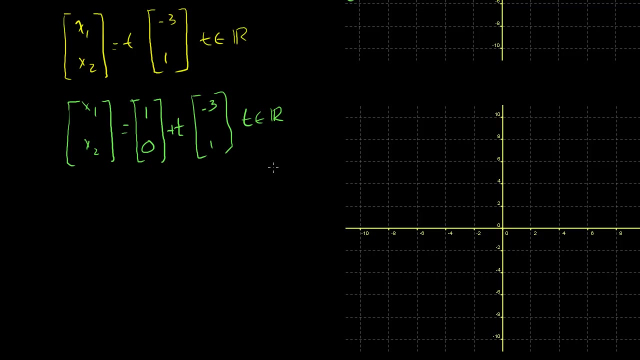 Let me copy and paste my two results. So I get, then I want to paste it. So those are my two results. Let me put my pen back on And now what I can do is I can graph it right here. So let's see. 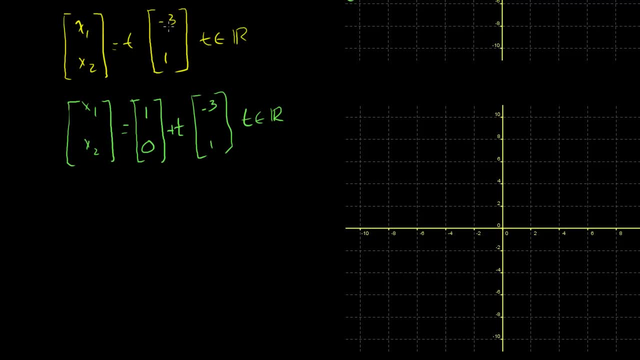 The solution set for that first equation is all the multiples of the vector minus 3, 1.. So the vector minus 3, 1 looks like this: It looks like that. That's the vector minus 3, 1.. But my solution set is all the scalar. 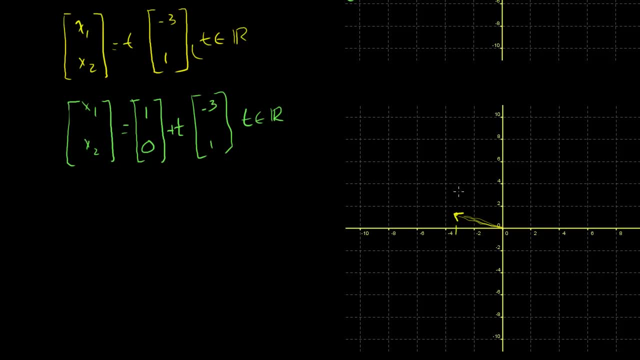 multiples of minus 3, 1.. This is a comma right here, Right? So if I just take all the scalar multiples of minus 3, 1, it's going to look like this: So if you take 2 times it, you're going to have minus 6, 2.. 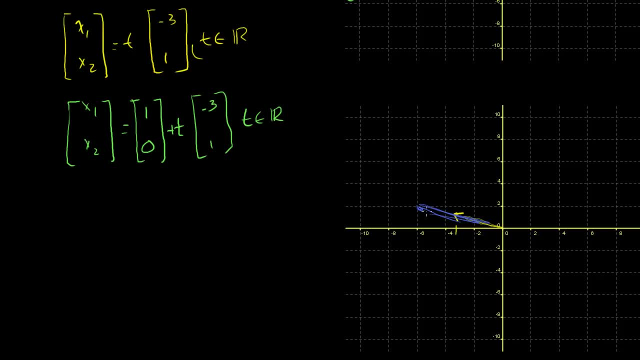 So you're going to get like that, So it's going to be all of these points right here. I wish I could draw it a little bit neater, but I think you get the idea. It's going to be a line like that. 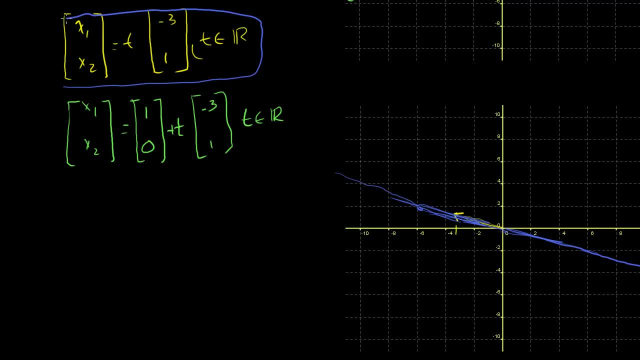 That is that solution set right there. And then what is this solution set right here? It's the vector 1, 0. So we go out 1, 0.. So that's there, Plus scalar multiples of minus 3, 1.. 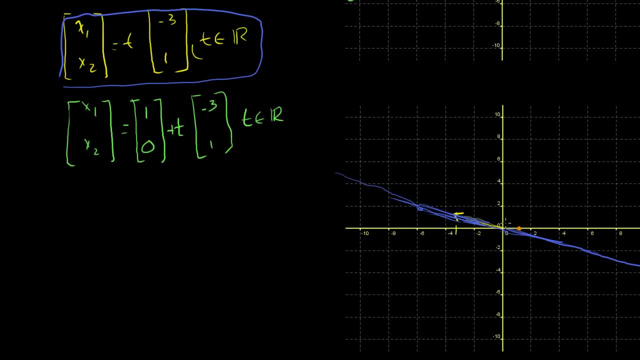 So plus scalar multiples of this. So plus scalar multiples. So if we just add one scalar multiple of minus 3, 1, we'll end up right there. But we want to put all the scalar multiples of it because we have this t right here. 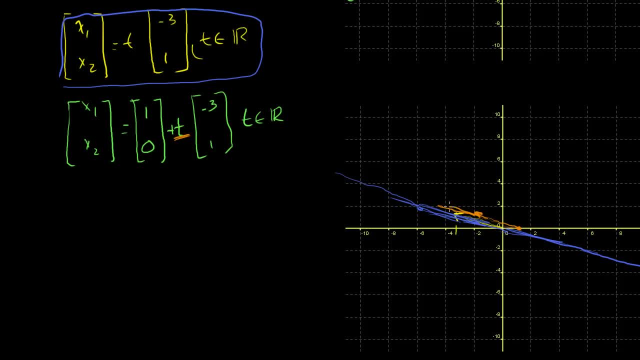 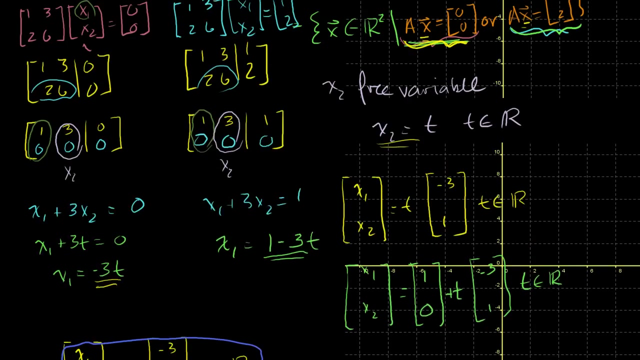 So we're going to end up with another line with the same slope. essentially, that's just shifted a little bit. It shifted 1 to the right. Now, why did we do all of this? Remember, what we wanted to find out is what were all of 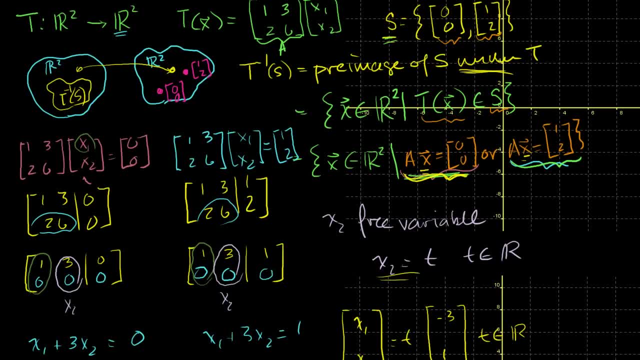 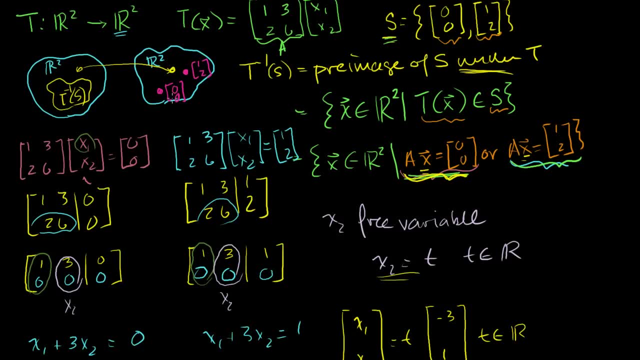 the vectors in our domain, that when we apply the transformation map to vectors, Map to vectors within our subset of our codomain Map to either 0, 0 or the vector 1, 2.. And we figured all of those vectors out by solving these. 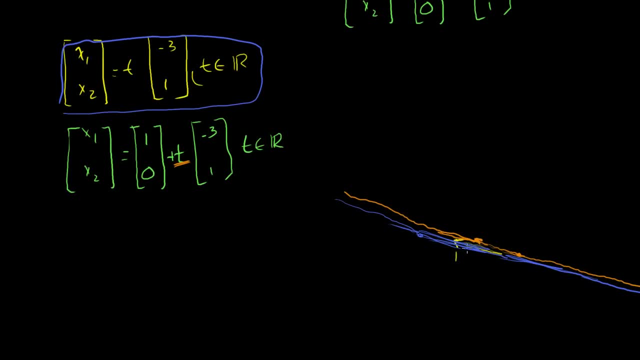 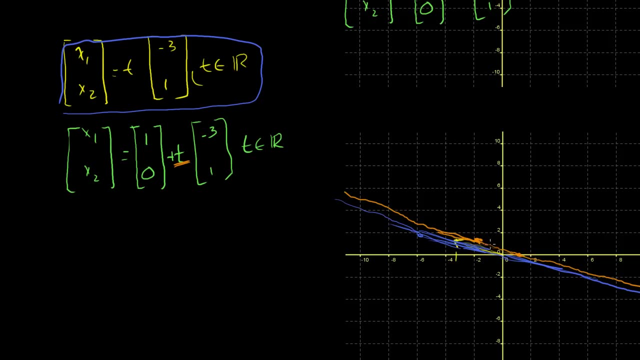 two equations And we were able to see that these two lines, when I turn my graph paper on, they map to the points. So when these guys, when you apply the transformation- I'll draw it all on the same graph- they map. when you apply the. 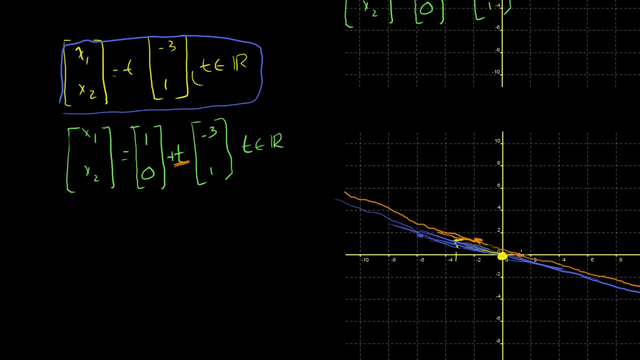 transformation to the points 0, 0 and to the point 1, 2.. Which was right here. So all of these points, when you apply the transformation, and actually all of the ones in the blue, they map to 0, 0.. 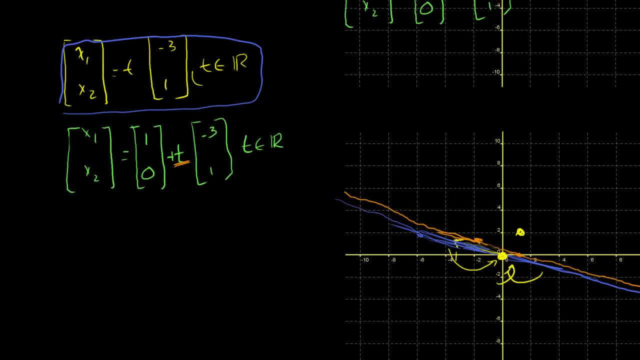 Because they solved this top equation. All the ones in orange when you apply the transformation map to the point 1, 2.. Now this blue line right here: this has a special name for it And I actually touched on it a little bit before, right. 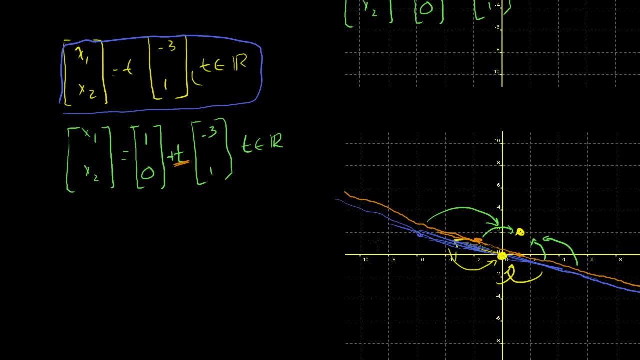 Everything in this blue line. right? If I call this set right here, I don't know. let's call it b for blue. this is the blue line. That's this set of vectors right here, Everything there. when I apply my transformation of those blue. 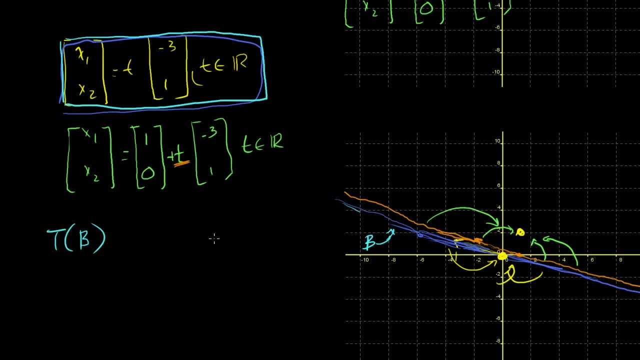 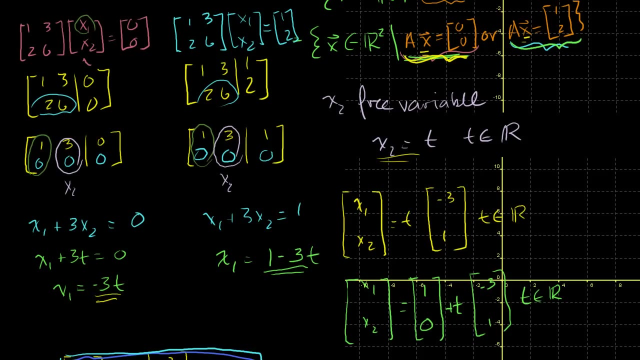 vectors. or if I take the image of my blue set under t, it all maps to the 0 vector. It equals the set of the 0 vector right And we saw that right there And I remember well earlier in the video I pointed out. 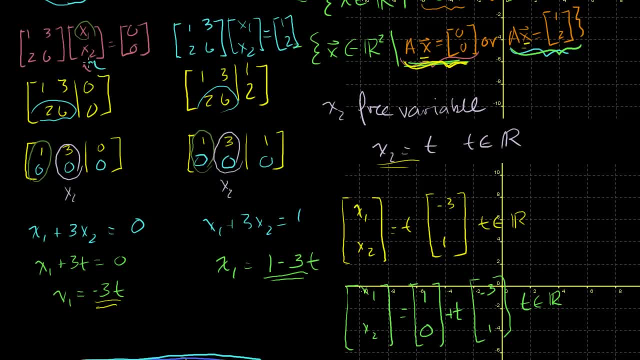 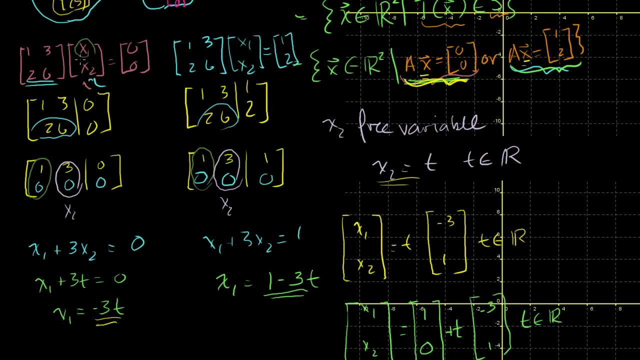 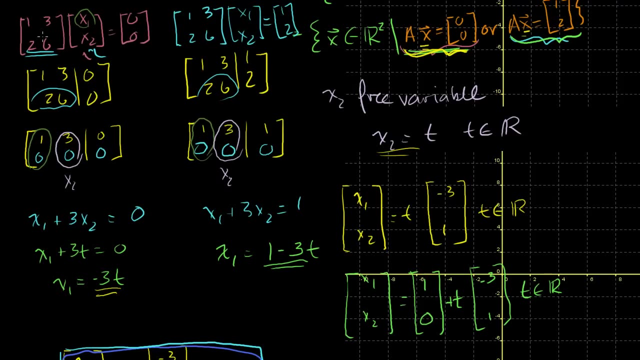 that. look this set right here. this is equivalent to the null space. right, The null space of a matrix is all of the vectors that if you multiply it by that matrix, you get 0. So the similar idea here is this: transformation is defined. 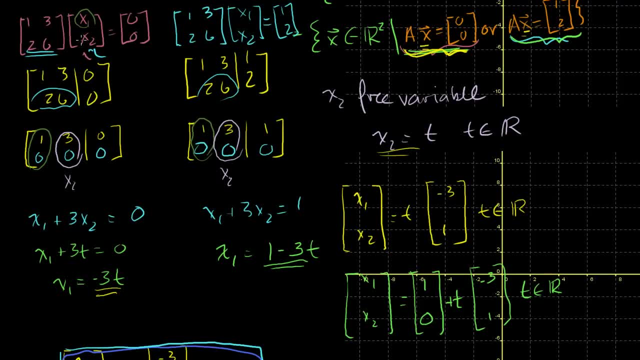 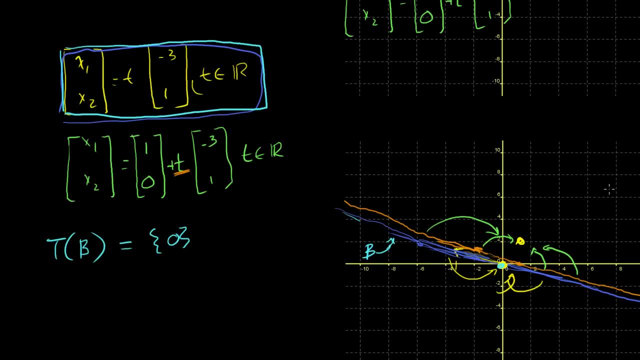 by a matrix. And we're saying: what are all of the x's? that when you transform them? when you transform them, you get the 0 vector. And so this idea, this blue thing right here, is called the kernel of t. 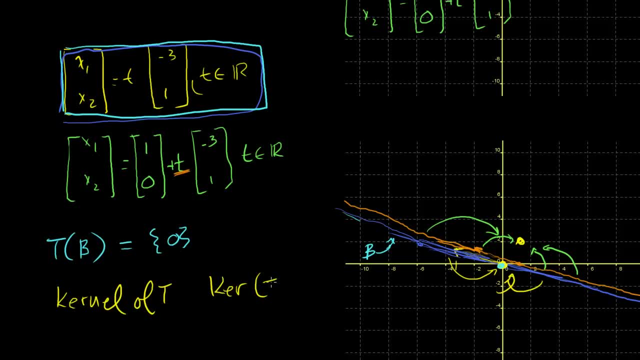 And sometimes it's written as just shorthand: k-e-r of t, And this, literally, is all of the vectors that, if you apply the transformation- let me write it this way- it's all of the vectors in our domain, which was r2, such that the 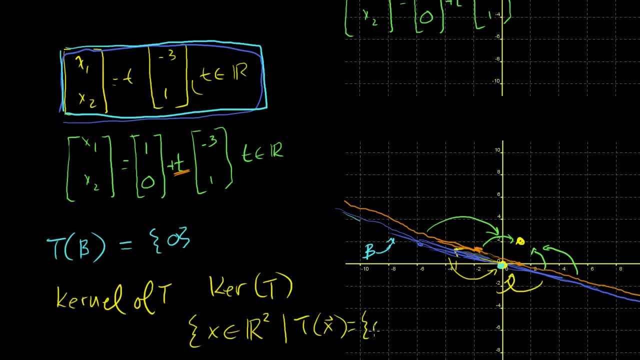 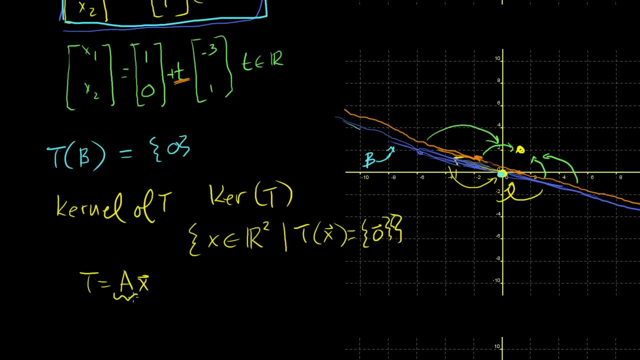 transformation of those vectors is equal to the 0 vector. This is the definition of the kernel. And if our transformation is equal to some matrix times some vector- and we know that any linear transformation can be written as a matrix vector product- then the kernel of t